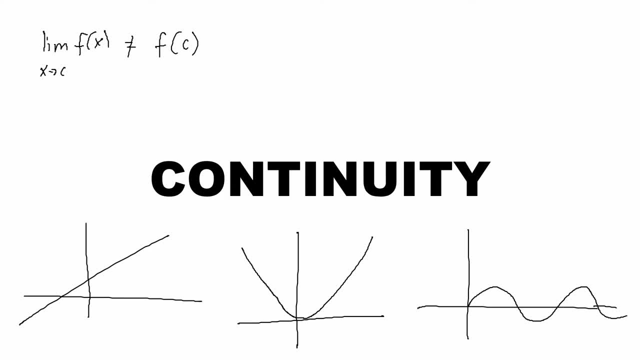 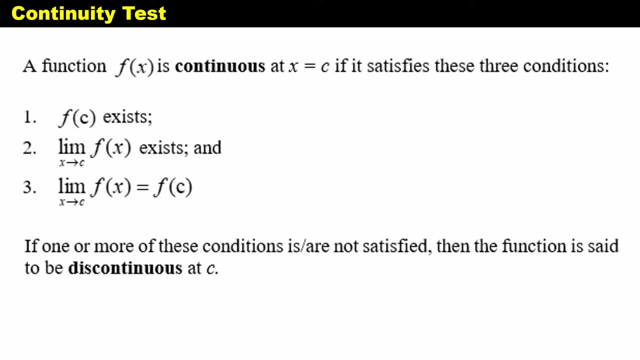 Now how do we know that the graph of a function is continuous? We have here a continuity test. A function, f of x, is continuous at x equals c if it satisfies these three conditions given: First, if f of c exists. Second, if the limit of f of x is continuous. 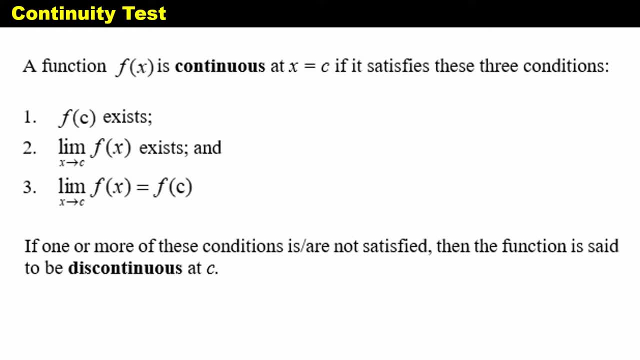 Third, if the limit of f of x as x approaches c exists. And last is, if the limit of f of x as x approaches c is equal to f of c. Now, if one or more of these conditions are not satisfied, then the function is said to: 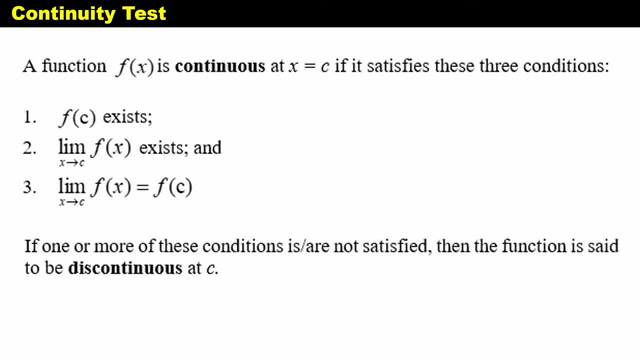 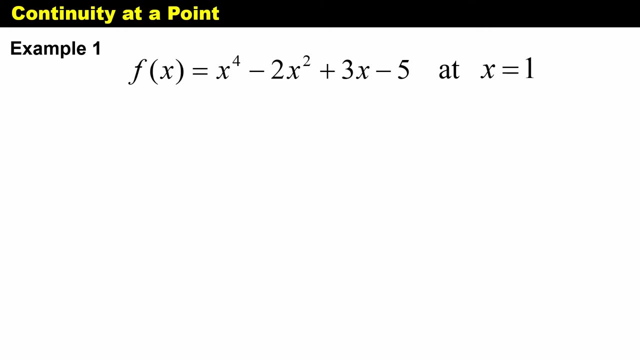 be discontinuous at c. So this is continuity at a point. Now let's have an example on how to identify if a graph of a function is continuous at a point. Say, for example: we have the function x to the fourth minus two, x squared plus three. 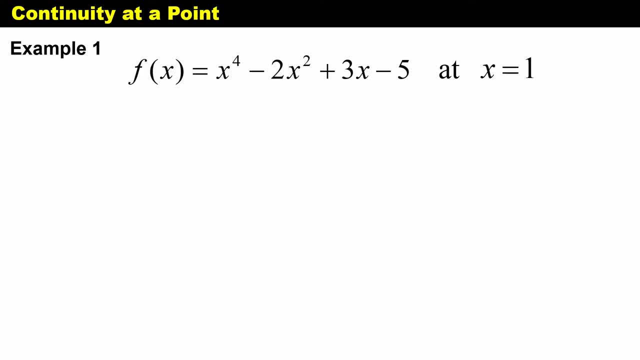 x minus five, and you are asked: if this function is continuous at x equals one, Now how do we solve this one? or how do we identify if this function is continuous at x equals one? Now, we will be using the three conditions that we have previously discussed. 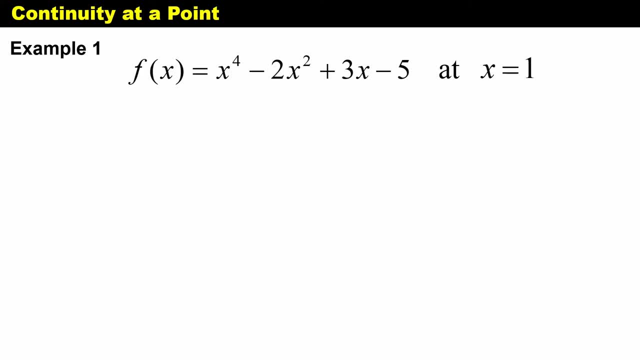 So the first condition is if f of c exists. Now, our value of c here is one. So let's evaluate f of one. So this becomes one to the fourth minus two times one squared plus three times one minus x squared. Okay, So this is one to the fourth. is one minus two times one, is two plus three minus five. 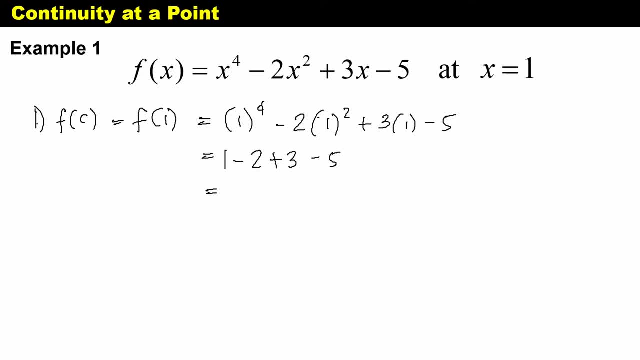 Now, simplifying this, we get negative. one plus three is positive. two minus five is negative three. So we already have our first condition. Now the second condition is: if f of c is continuous at x equals one. So we already have our first condition. 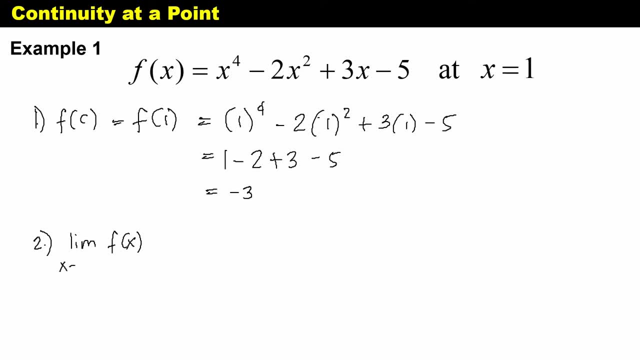 Now the second condition is, if f of c exists, The limit of f of x as x approaches c exists. Now we will be solving for the limit of x to the fourth minus two x squared plus three. x minus five as x approaches one. So by substitution we have one squared minus two times one squared plus three times one. 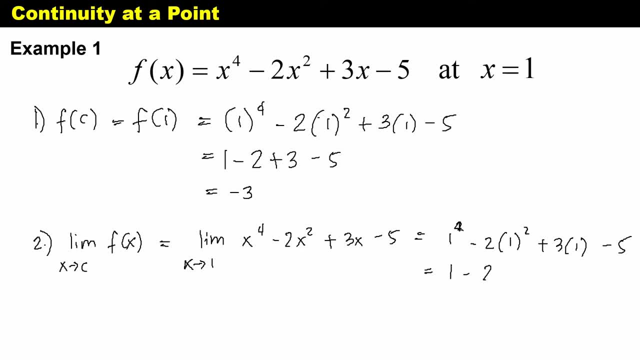 minus five. This is one minus two plus three minus five. One minus two is negative. one plus three is positive. two minus five is negative three. Now both our first and second condition exist. So let's now move on to our third condition, That is, if your f of c is equal to the limit of your f of x, is x approaches c? 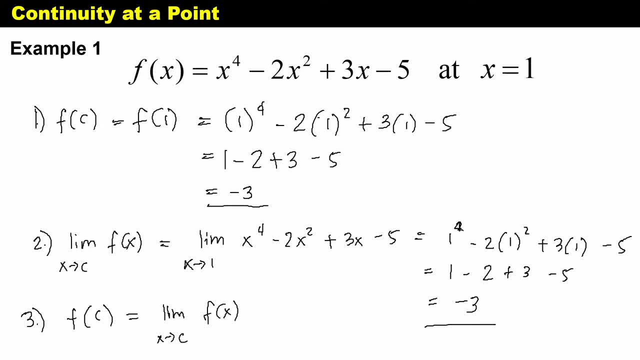 So we want to find out the third condition, That is, if your f of c is equal to the limit of your f of x. is x approaches c approaches C? now the value of our f of C is negative 3. then the value of our 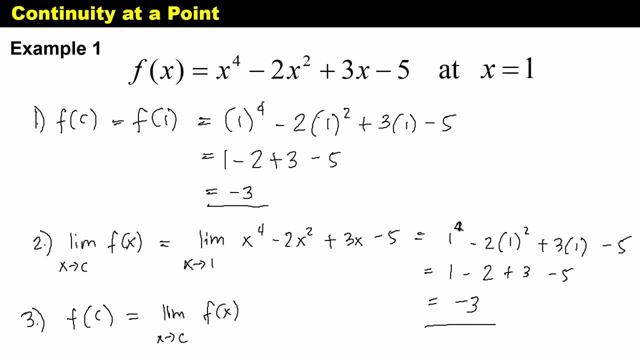 limit of f of X as X approaches C is also negative 3. therefore this graph satisfies our third condition. now, what we have discussed earlier is the graph of the function is continuous if it satisfies the three conditions given. now it's satisfied that f of C exists. the limit of f of X as X approaches C exists. 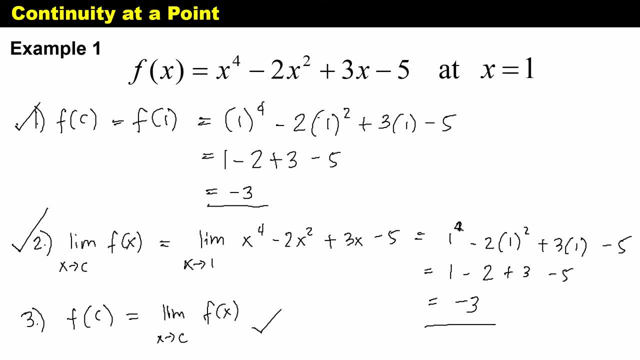 and since their values are equal, then it satisfies also the third condition. now it's satisfied the three given conditions. therefore, this function f of X equals X to the fourth. minus 2x, squared plus 3x minus 5, is continuous at X equals 1. 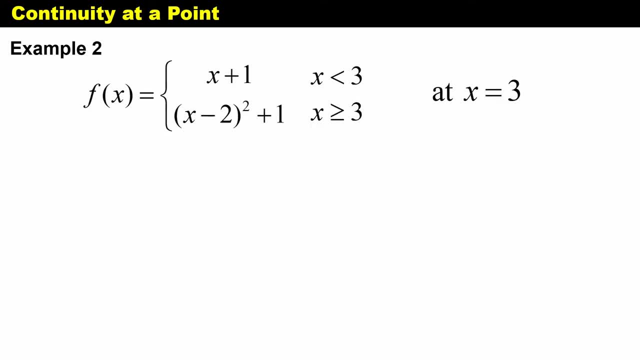 now let's have another example. say we have a piecewise function: f of X equals X plus 1 if X is less than 3, and X minus 2 squared plus 1 if X is greater than or equal to 3 at X equals 3. now we'll be identifying if these function or this. 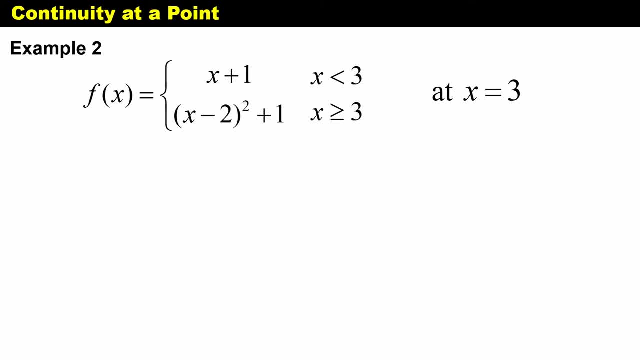 piecewise function is continuous at X equals 3 equals 3. now let's solve for the first condition, which is the f of C. f of 3 is equal to what. now we will be deciding which function will we use in solving for f of 3. now, in the conditions given, if X is greater than or equal to 3, you 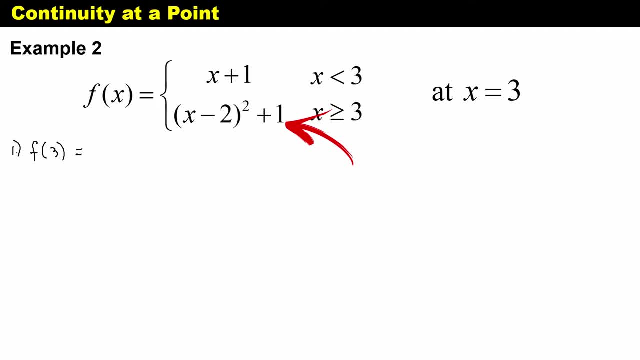 will use this function. therefore, we will make use of the second function. this becomes 3 minus 2 squared plus 1. now, simplifying this one, this is 3 minus 2, which is 1. 1 squared is 1 plus 1 equals 2, so it. 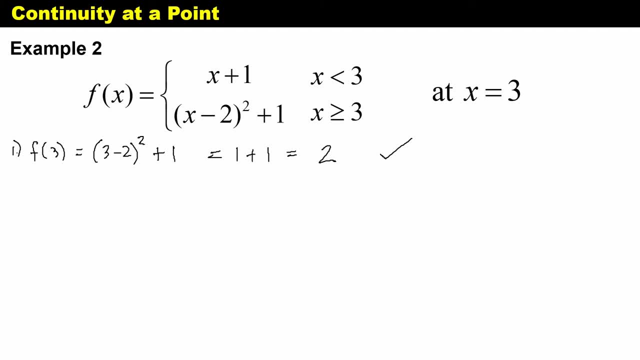 satisfies our first condition that f of 3 or f of C exists. since this is not undefined, so it exists. now let's solve for the second condition. second condition says that the limit of f of X as X approaches C exists. now let's try to solve for the limit of this one limit of this function. 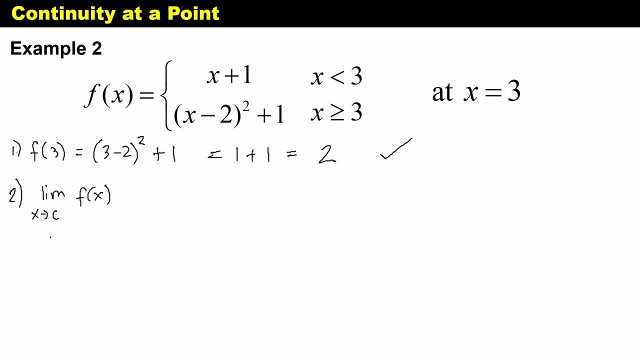 as X approaches C. since this is a piecewise function, it's better that we solve this one by looking at the one-sided limits of this function. so let's solve first the limit of f of X as X approaches 3 negative or values less than 3. now the condition. 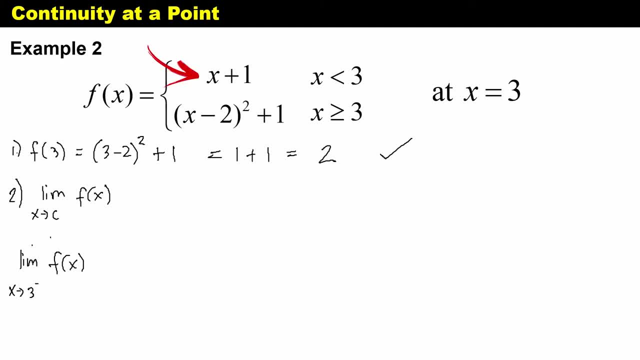 says that if X is less than 3, we will make use of this function. so we will use X plus 1. so substitute 3, 2x and then plus 1. therefore the limit of f of X as X approaches 3 negative, is 0. 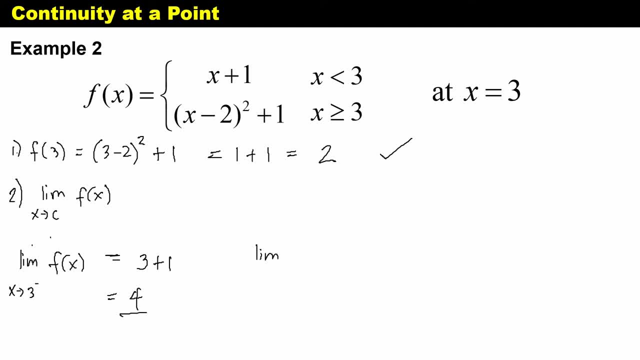 4. now let's try to solve for the limit of f of X as X approaches 3 positive, or values from the right of 3. now, values from the right of 3 are, of course, greater than 3, so we will make use of this second. 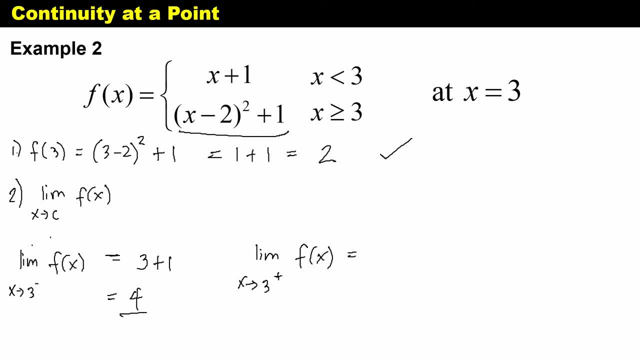 function. so if we substitute 3 to the function, this will become 3 minus 2 squared plus 1, and we know that 3 minus 2 is 1, squared is 1 plus 1 is 2. now the limit of f, of X, as X approaches 3. 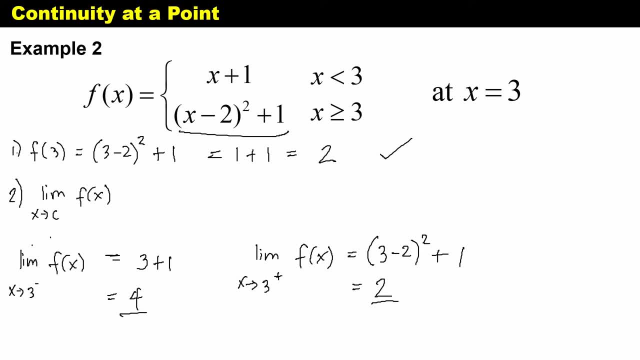 positive is: 2 limit exists if, and only if, the one-sided limits are equal. now, since your one sided limits are not equal, therefore, the limit of f of X as X approaches 3 does not exist now. it does not satisfy the limit of f of X as X approaches 3. it does not satisfy the limit of. 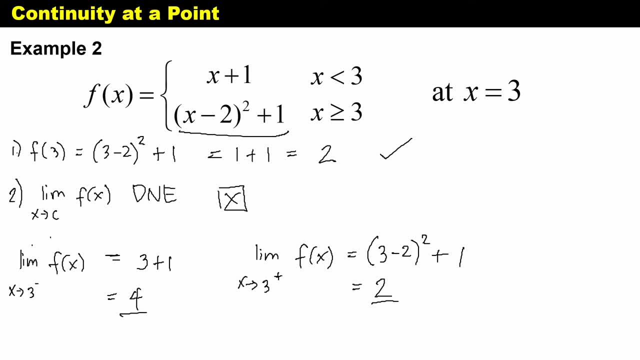 second condition now, as what we have discussed earlier, if one or more conditions are not satisfied, then the function is not continuous at a point. therefore, the function f of x equals x plus 1 if x is less than 3 and x minus 2 squared plus 1, if x is greater than or equal to 3, is not. 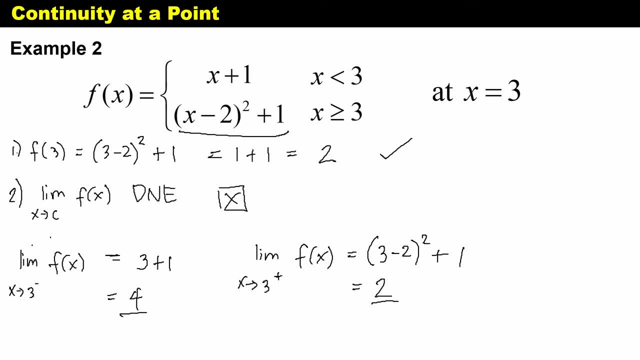 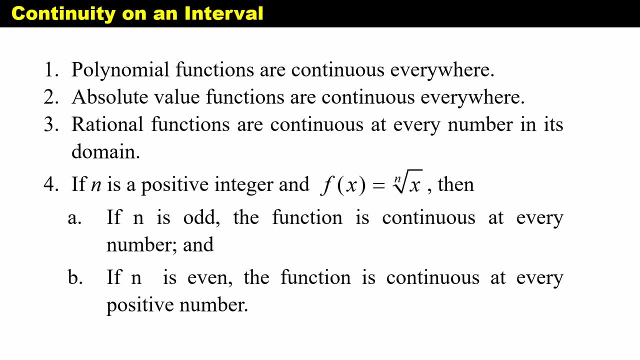 continuous at x equals 3.. now we also have this continuity on an interval. now, what is continuity on an interval? the same, with the concept of continuity at a point, you can say that the graph is continuous at every point on an interval, if you are able to draw the graph of the function without 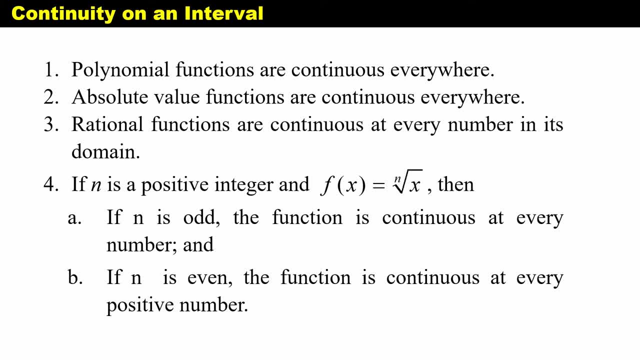 lifting your pen or without being interrupted by these continuities like a hole or a break or asymptote. now, before we move to our examples, let us have first these known facts about continuities of functions on intervals. first is that polynomial functions are continuous everywhere. second, absolute value functions are continuous everywhere. third, rational functions are: 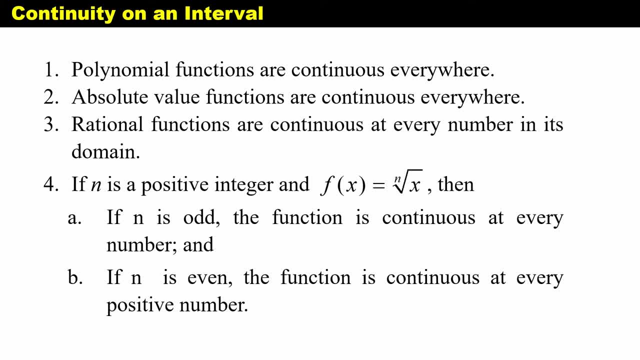 continuous at every point or every number in its domain. and the fourth is if. if your function is a radical function, if n is a positive integer, in that your function is equal to the nth root of x, then if n is odd, the function is continuous at every number. 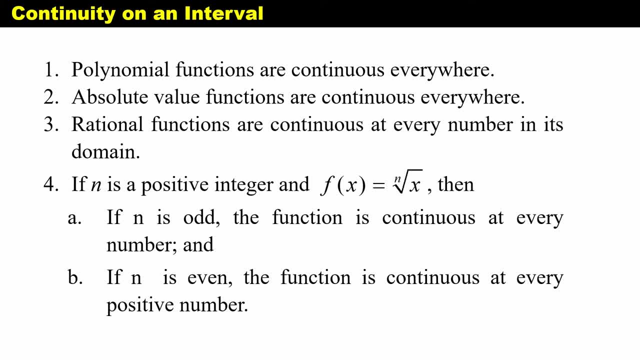 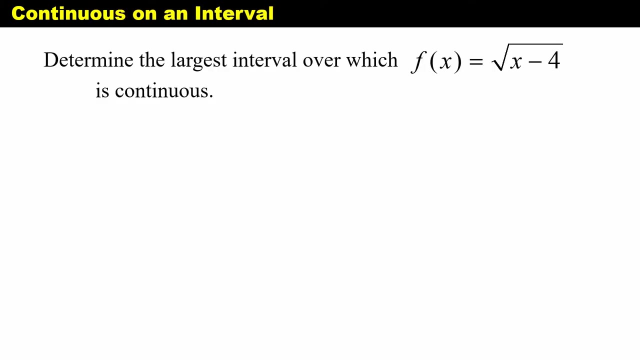 and if n is even, the function is continuous at every positive number. now, these are the known facts about continuities of functions on intervals. now, we will now move on to our examples and apply these known facts about continuity on intervals. let's move to our first example. determine the largest interval over which f of x. 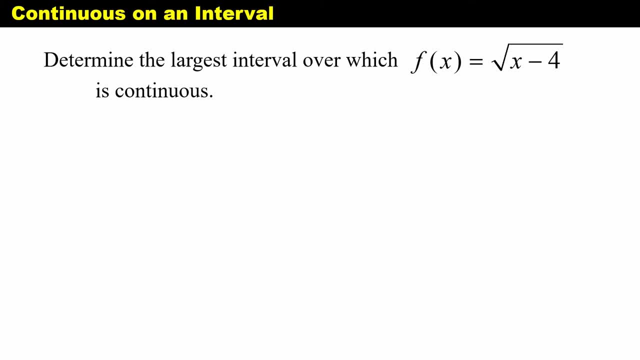 equals. the square root of x minus 4 is continuous. now notice that the index of our radical function is even, since the index is 2, so it's even meaning the function is continuous at positive numbers only. this means that a radical should be greater than or equal to zero. so we write a radical x minus 4, greater than or equal to zero. 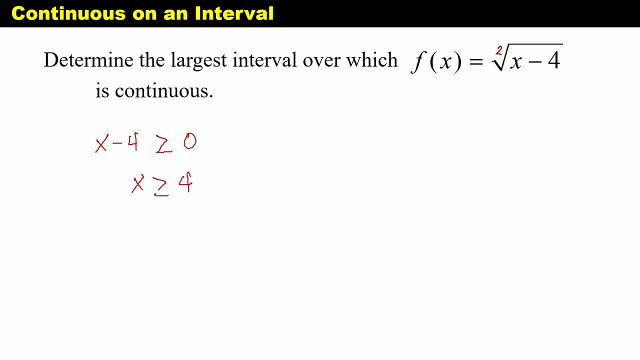 therefore, our x should be greater than or equal to positive four. now remember that, since we cannot make a radical negative, the function of or the function is only continuous for x and we can't make this negative, so we can write an values greater than or equal to positive 4, thus the largest interval over which this function is. 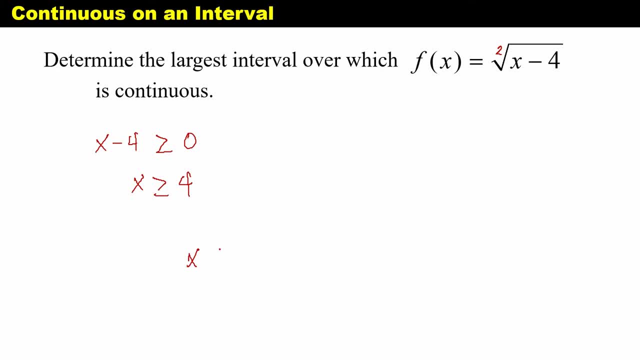 continuous is. X is an element of an interval half open on the right from positive 4 to positive infinity. this is our final answer. now the seven of the example we have: F of X equals X plus 2, all over X squared minus 1. now remember that the domain of this function 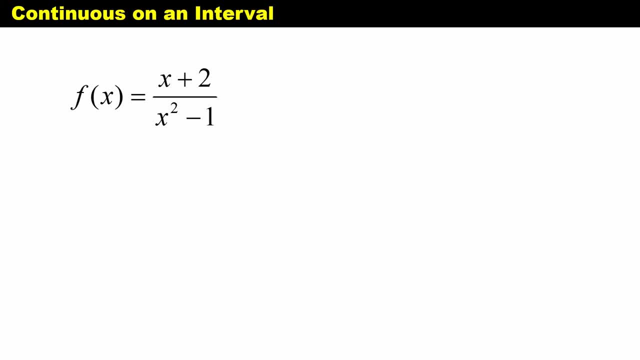 is the set of all real numbers, except for values that can make our denominator equal to 0, a. so so let us try to look what are the values that could make our denominator equal to zero. so let's focus on our denominator. so we have x squared minus one, and we know that this is factorable.